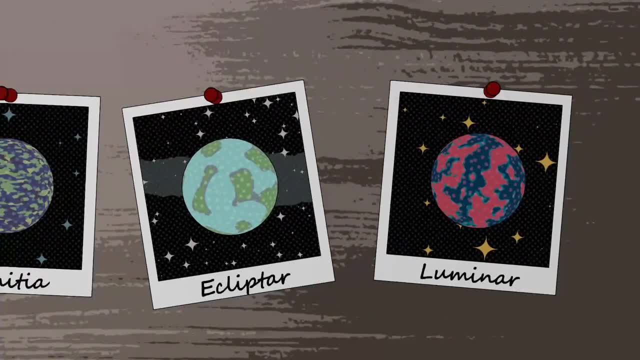 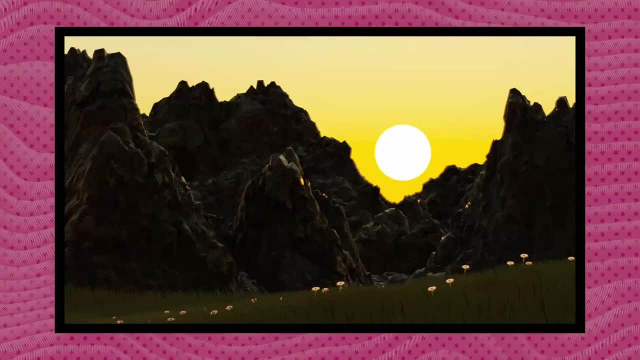 To get a better understanding, let's take a look at an example. In this image we can see lots of fine details. For example, there's a field of grass and flowers in the foreground and the background has a very detailed mountainscape. But there's still a bright star in this scene. 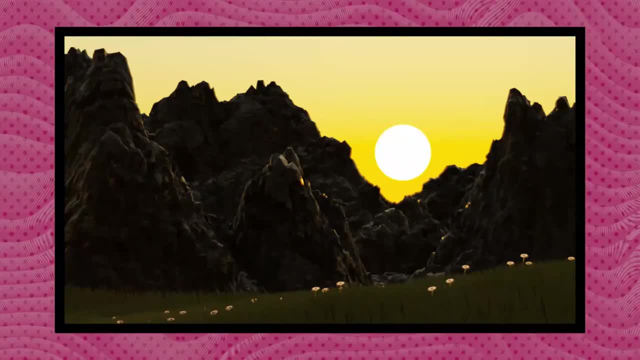 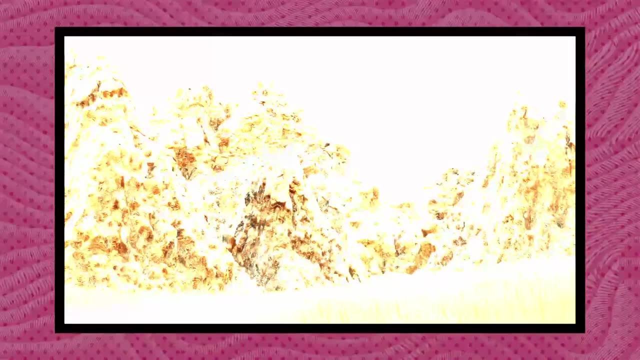 So if we aren't careful about how we take the photo, we can end up with something that looks like this, where all of those fine details are washed out by the star's light. You can imagine how, if we're trying to look at planets that are only dimly lit, it would be nearly 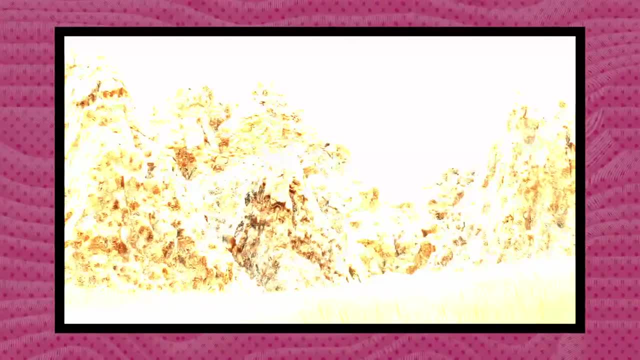 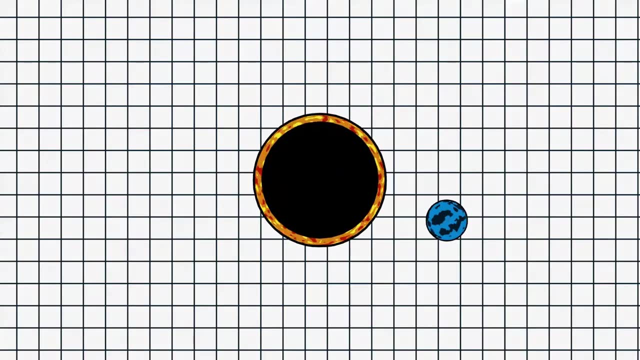 impossible to find them in images like this. So how do we actually fix this issue? If we're looking at a star, then we can place a filter over our camera to block out some of its light. This is a very simple way to get a better understanding of how a star looks like. 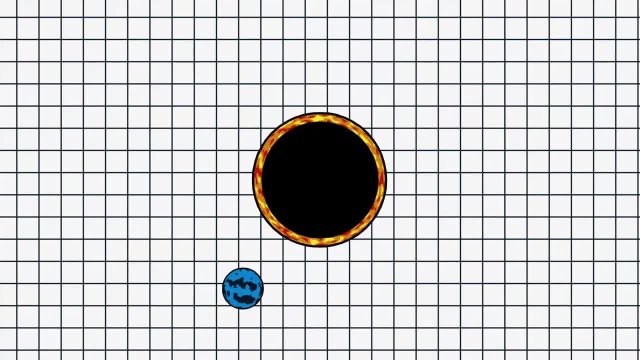 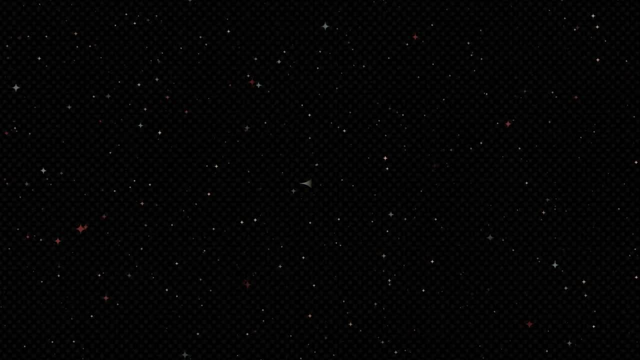 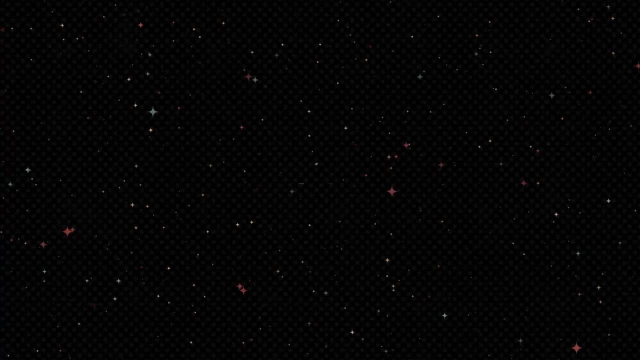 This makes it easier for us to identify any planets in the image, especially if they're orbiting close to the star and are well lit. Looking up at the night sky, you may notice stars dimming and brightening again On Earth's surface. this is usually caused by light bouncing around in the atmosphere, But we can still. 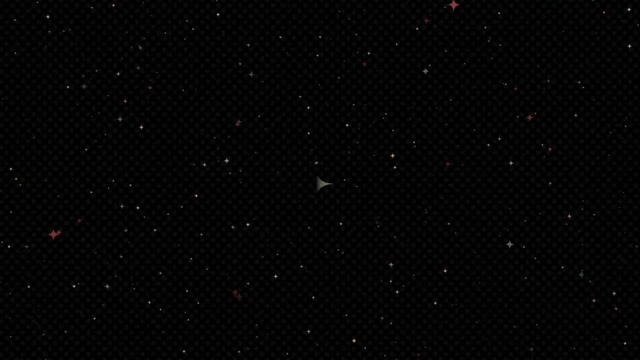 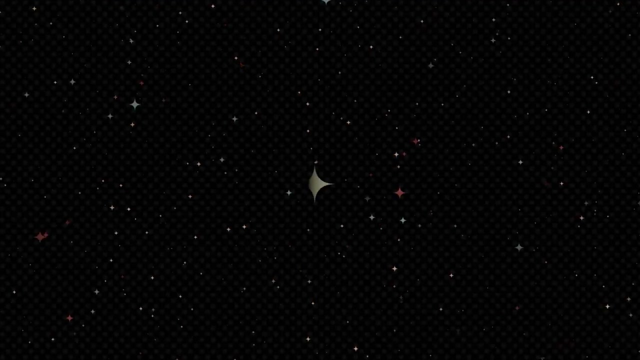 see this dimming when we look at stars that are dimming and brightening again. We've been looking at stars for a long time from space telescopes. This could be happening for many reasons, like the stars' natural aging. However, in a particular case, where 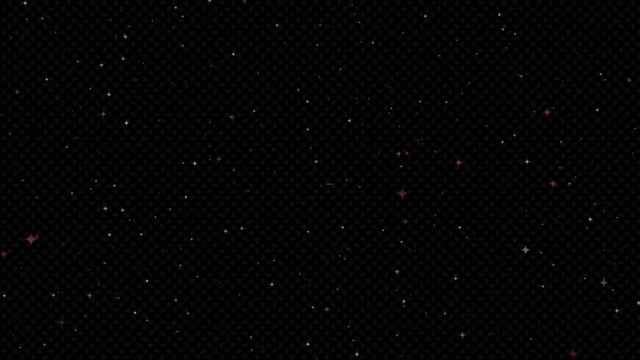 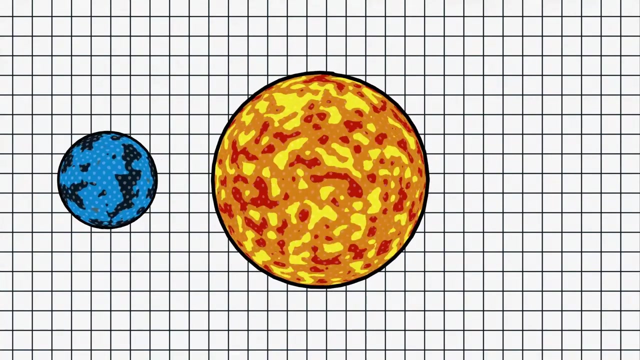 the time between these dimming events is constant. we might be looking at something called a transit event. Here a planet passes in front of its host star, blocking a large amount of its light, And much like how the Earth takes a regular amount of time to orbit around. 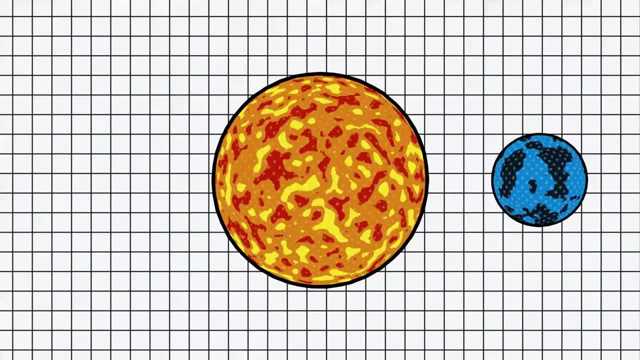 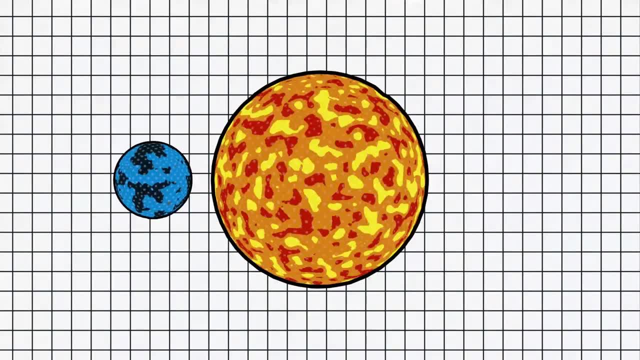 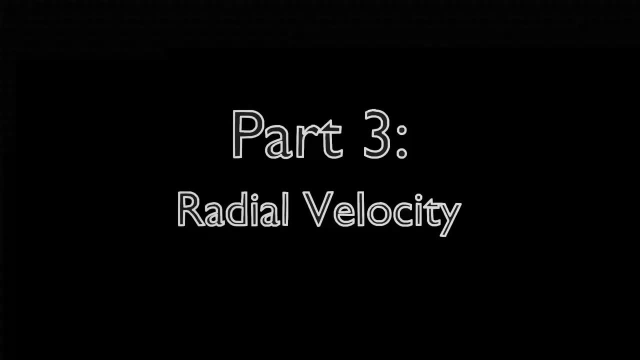 the Sun. these planets take a constant amount of time to orbit their host stars. This is what causes the frequent periodic dimming effect from before. So long as a planet is large enough, a space telescope can measure these dips in brightness to find them. If you've ever stood by a busy road, you've probably heard this sound. Notice how the car's horn dropped from a higher pitch to a lower one. This is an example of the Doppler effect, And it happens every single time. This is an example of the Doppler effect, And it happens every single time. And it happens. 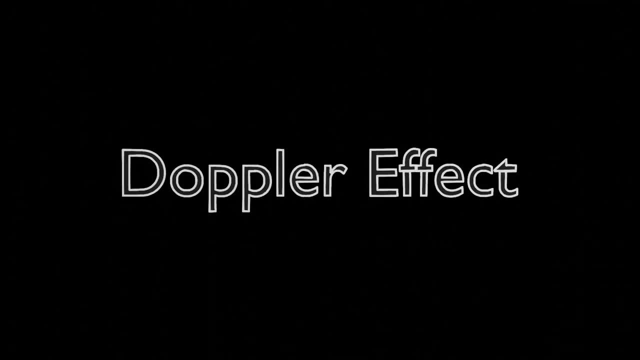 any time the waves are emitted by a moving object, because the waves build up differently on different sides of the emitter. To understand why, though, let's look at an example. Here we can see that the waves are much more compressed on the right side of the emitter than on the 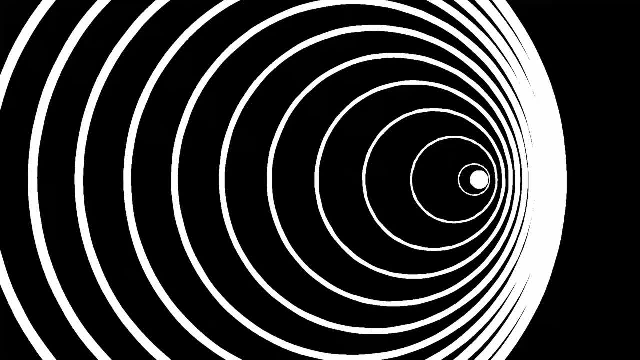 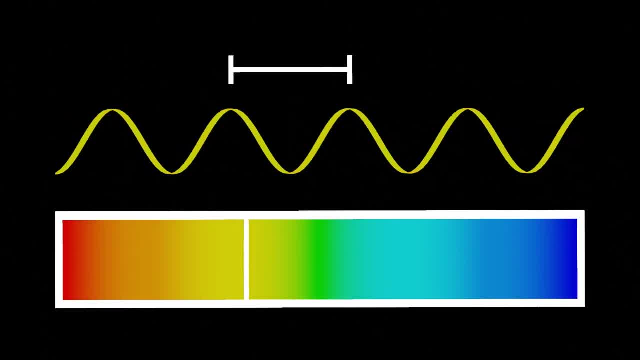 left. This difference in compression causes a car's horn to sound different as it passes by you. But this effect applies to more than just sound. Light also behaves as a wave, meaning that if an object is emitting light and moving, it will also be emitting light. This effect applies to more than just sound. Light also behaves as a wave, meaning that if an object is emitting light and moving, it will also be emitting light. This effect applies to more than just sound. Light also behaves as a wave, meaning that if an object 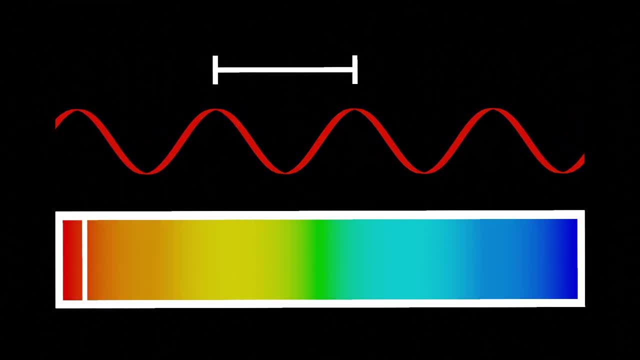 is emitting light and moving it will also be emitting light. The light they emit can compress and expand. Additionally, the light's compression affects how we perceive its color. Light waves appear bluer when compressed and redder when broadened. So if we know what a star should look like at rest, we can figure out how it's moving. 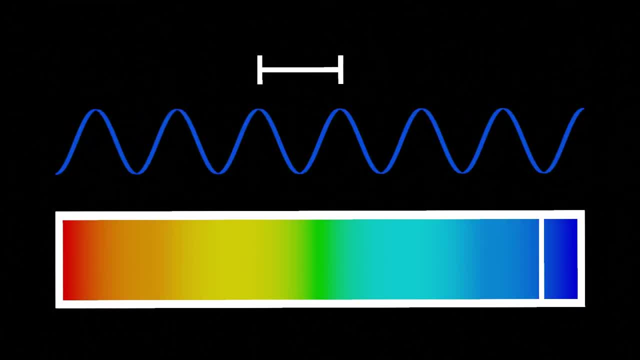 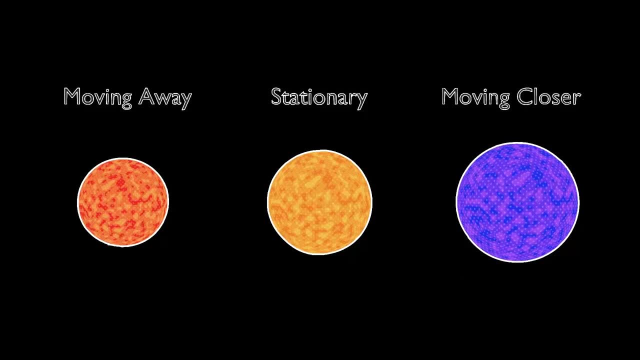 by observing its long-term color. For example, a star moving away from us would look redder than at rest, and a star getting closer would appear bluer. But these are still similar, simple, one-dimensional motions. And how does this relate to finding planets? Well, 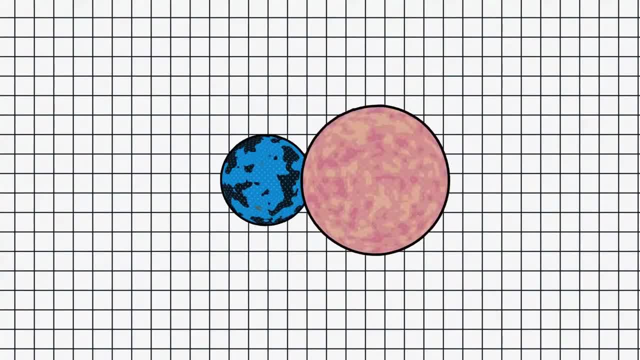 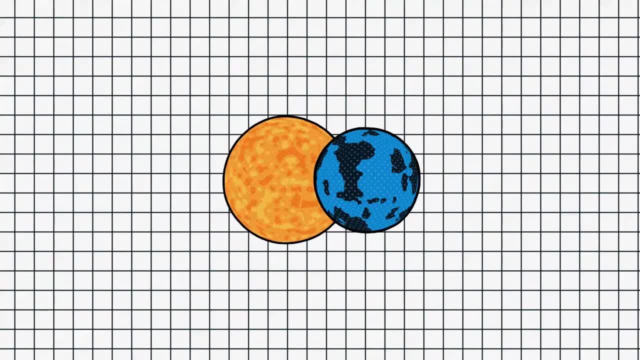 if a planet is massive enough, then it can cause its host star to move in a noticeable circular pattern. When looking at this star, it periodically shifts towards redder and bluer lights. The effect here is a dramatic exaggeration of what we would actually see. 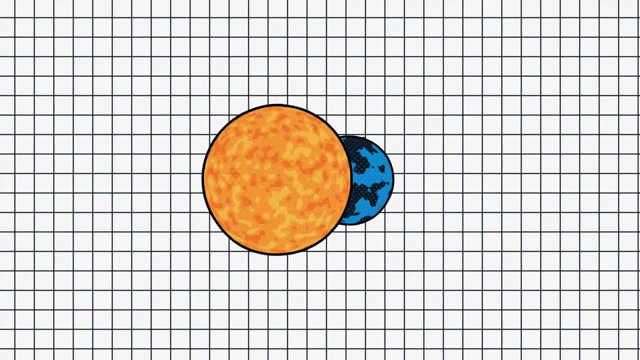 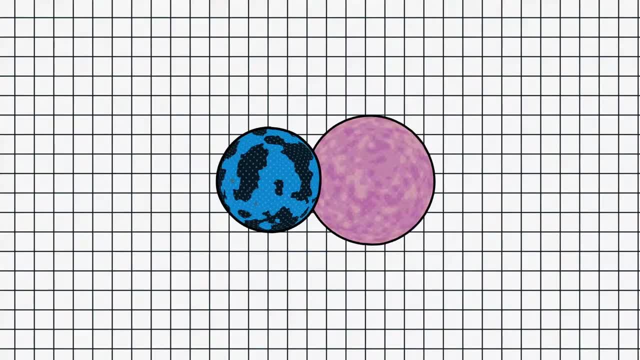 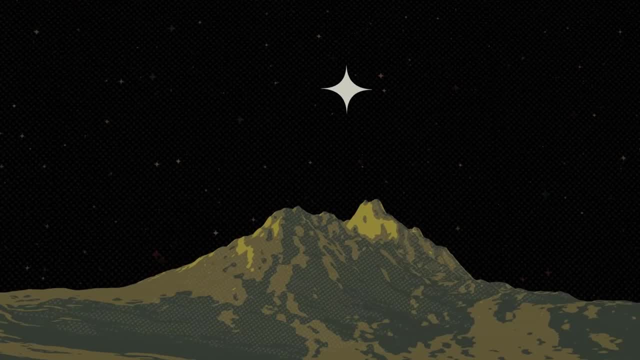 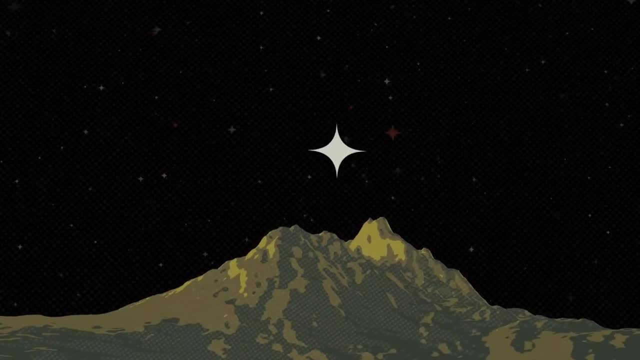 but it still demonstrates how, by observing these periodic color changes in a star, we can infer that a massive object is orbiting it. One night you look at the stars and notice a bright object moving in a circle. To confirm it's not a plane or helicopter, you are confident it is a star. What could be causing? 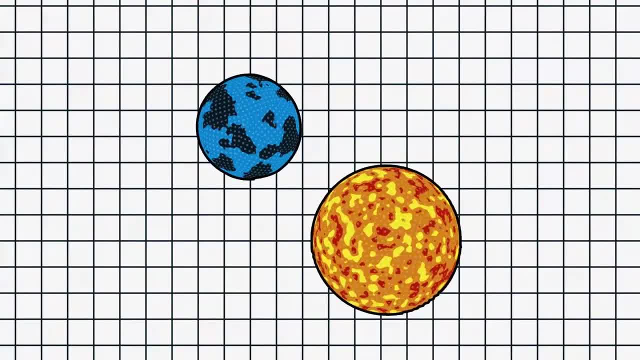 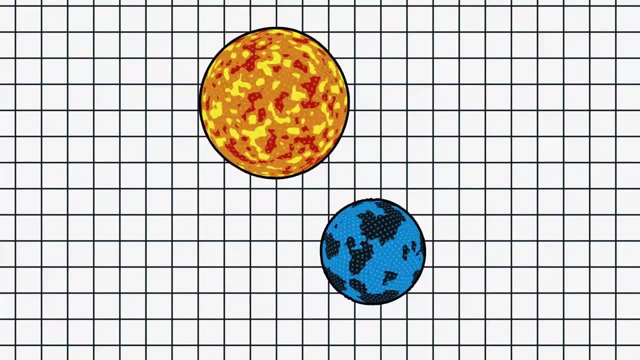 it to move like that. Remember, if a planet is massive enough, it can cause its host star to move in large circles. But unlike the radial velocity method, the star's light isn't changing color because its motion doesn't bring it closer or further ahead in the circle. So if the star's light is growing, this means that it's moving in circles. So what is the reason the planet is moving as large as its host star? Well, it's not that the star's light is changing color, because the 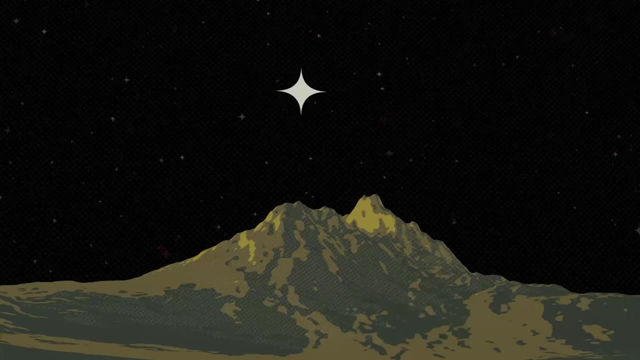 closer or further to us Instead. astrometry relies on tracking a star's position over a long time, But every star in the sky is unimaginably far from us, so even large circular motions would look nearly imperceptible. Even here, the star's movement is too large, Until. 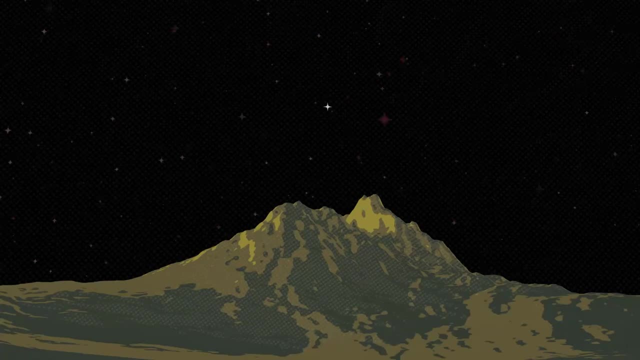 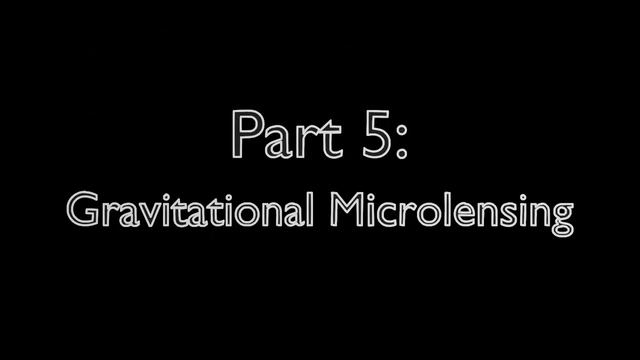 significant improvements are made in our observational instruments, this method is unlikely to find widespread use. You, me and nearly everything else on Earth has something in common: Gravity pulls us toward the ground. If I were to throw a ball, it would still move in the same direction. 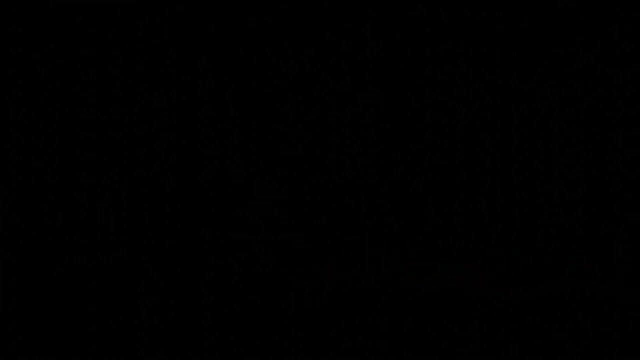 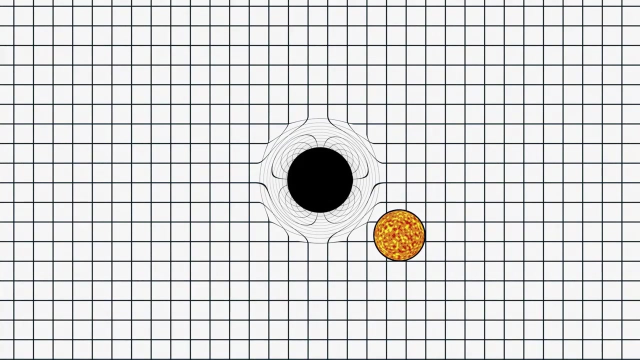 I threw it, but it would keep falling back to the ground. Shockingly, light can also be redirected by gravity. When light passes by massive objects, the light's path can warp and cause some weird behavior. For example, black holes can warp light so much that you 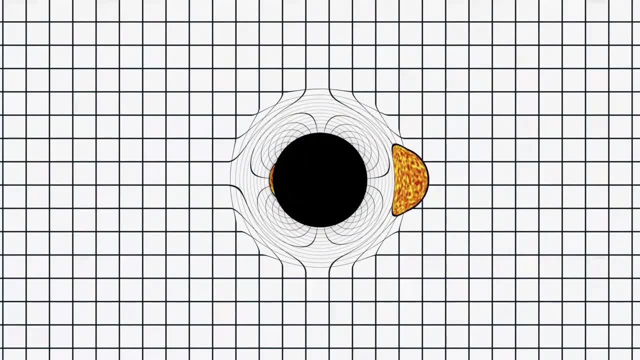 can see objects on the other side. Not only that, but this warping magnifies the brightness of these obscured objects. In the case of a star, we would see its brightness increase as it passed behind the black hole and decrease once it moved further away. This weird behavior is called gravitational lensing. But what? 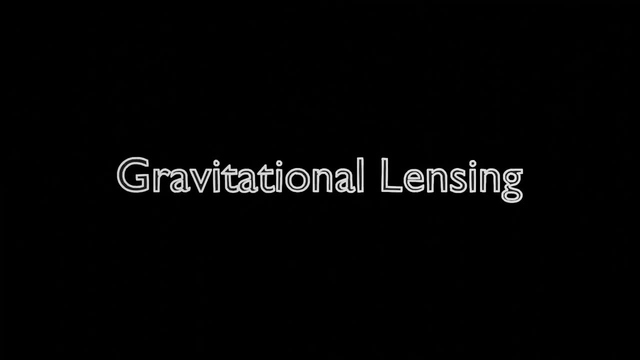 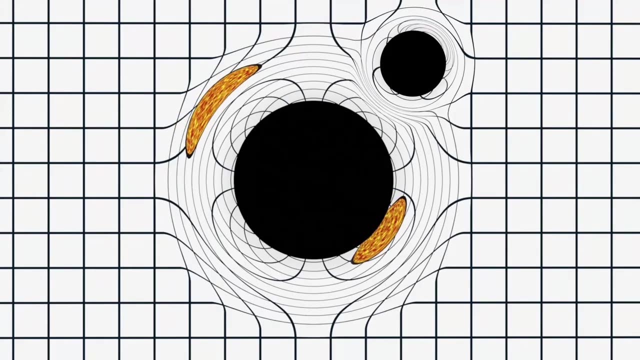 would happen if we had another black hole orbiting around the larger one? The star's light would still magnify like before, but the smaller black hole would cause a second peak in the star's brightness. This second peak tells us that another object is orbiting. 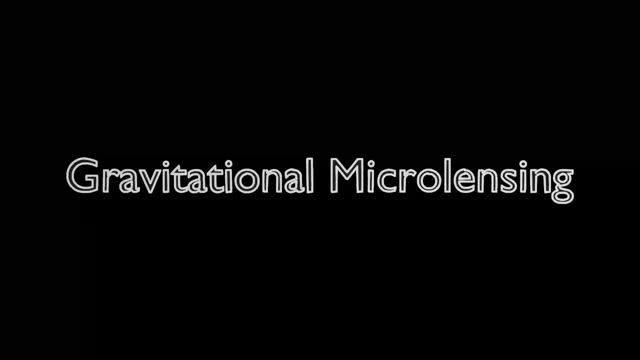 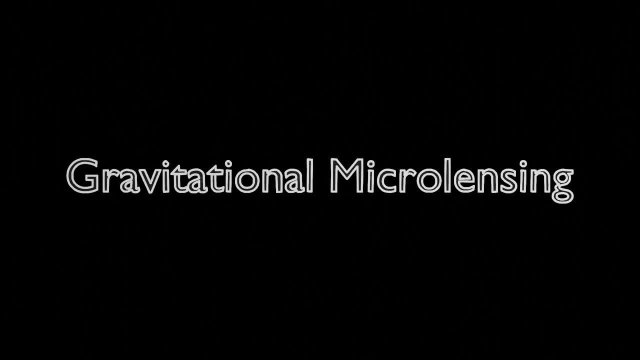 the larger massed and is called gravitational microlensing. We can replace these black holes with any other massive object, like stars and planets. So if we see a star's brightness peek twice as it passes behind another star, we may have just detected a. 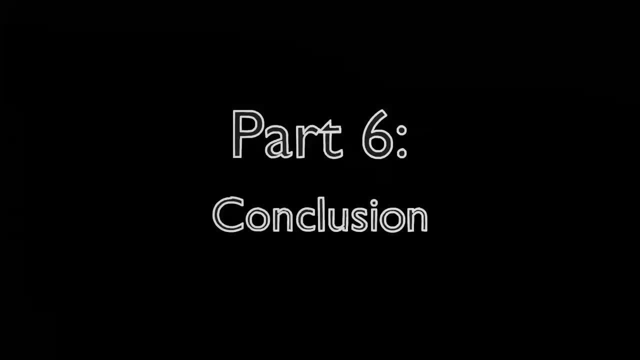 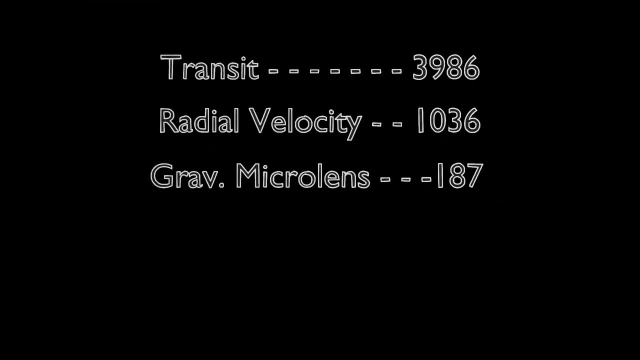 planet. If there's one thing to take away from this video, it's that there are many unique ways that planets are discovered, But they aren't all equally successful. The vast majority of exoplanets have been discovered using the radio velocity and transit methods. These numbers are pulled from the NASA Exoplanet. 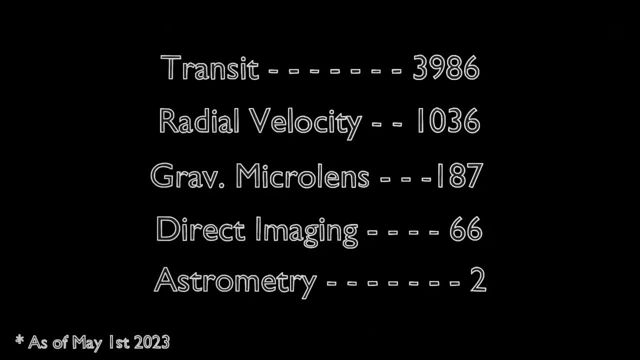 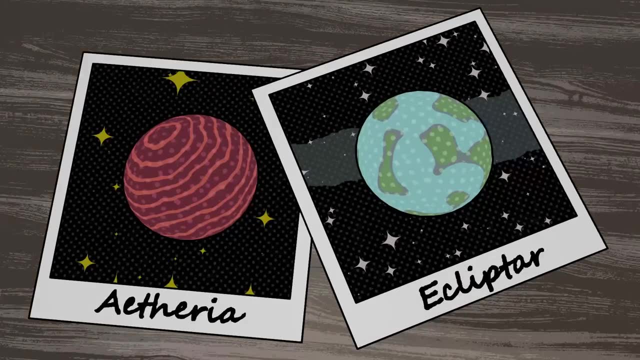 Archive and a link will be provided in the description. However, this isn't the complete picture, as many of our space telescopes are designed for those methods. Future space telescopes, like the Nancy Grace Roman Space Telescope, will focus on other methods like gravitational